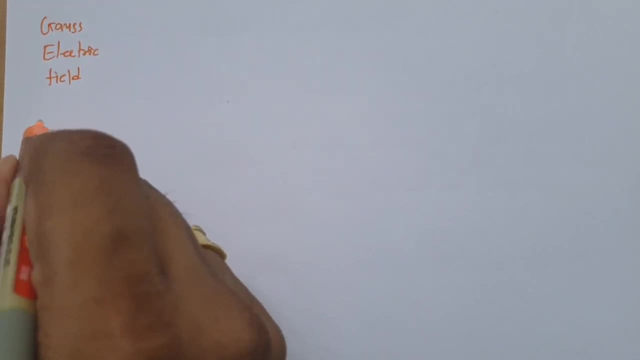 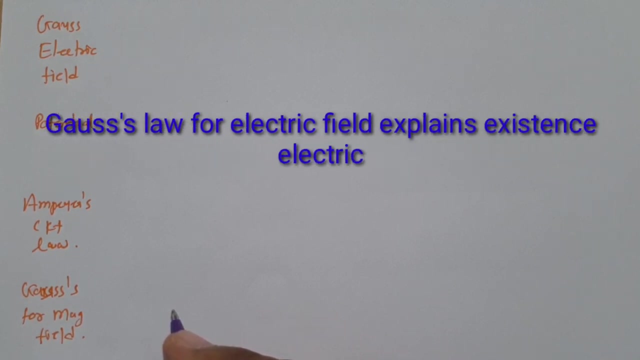 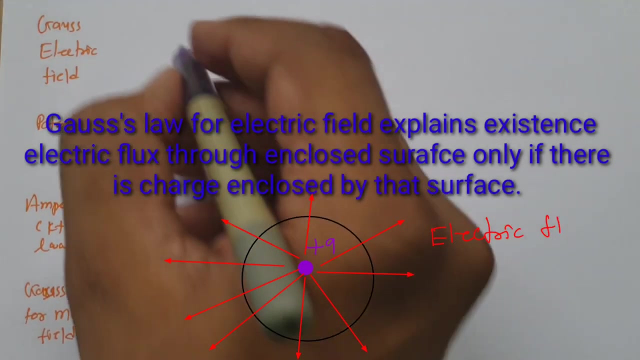 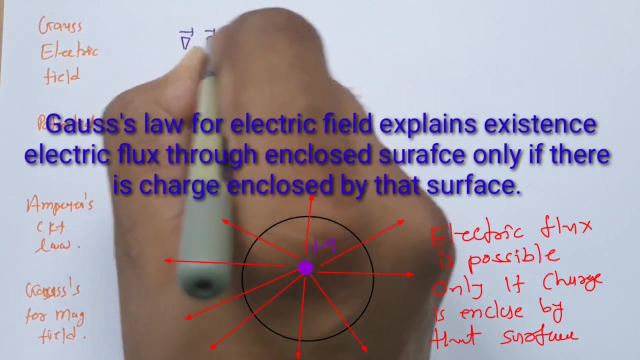 Then second equation That was there based on potential. third equation that is there based on ampere circuit law. and fourth equation that is there based on Gauss's law for magnetic field. Now see Gauss's law for electric field, Right? So that explains you. existence of flux is there for enclosed surface only if it enclose charges, Right? So first here I'll mention differential form. So differential form that is del dot d, that is equals to rho v. 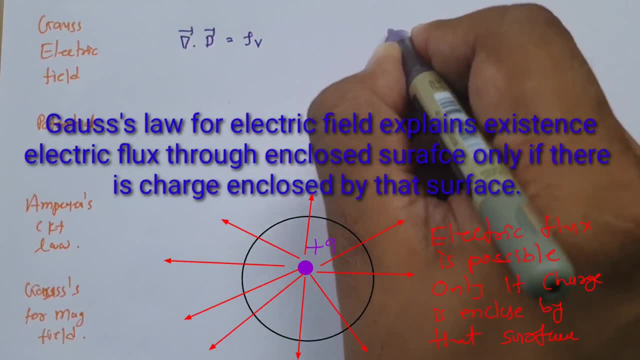 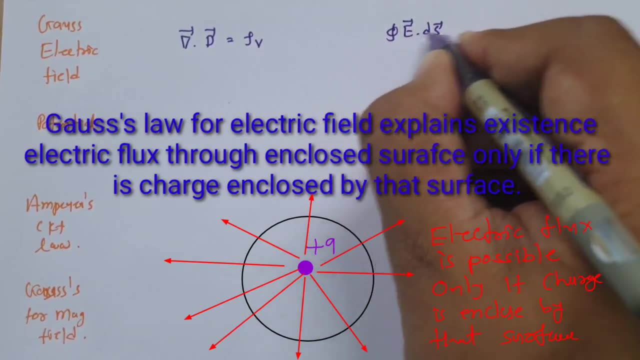 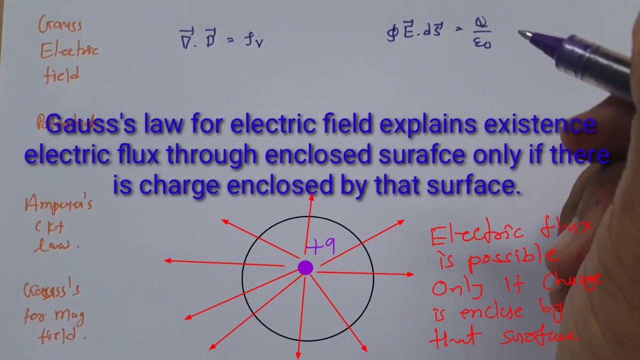 And this is integration E ds Right And integral form. that is integration E ds Right, That for enclosed surface integration E ds that is equals to q by epsilon zero Right. So this is how Gauss's law for electric field is been there. 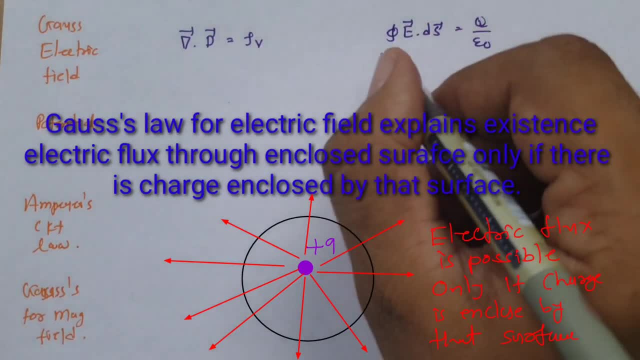 So what it explains? it explains electric flux for enclosed surface And this is like 0. So what will be the consequence? So this is what is the consequence: legenbox, that 소 like să س hazards. you have to imagine this half petri axが까요. 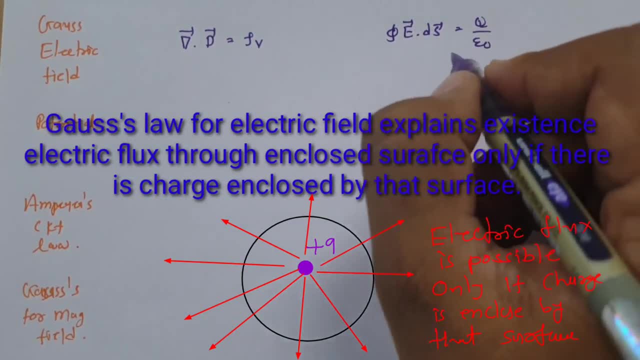 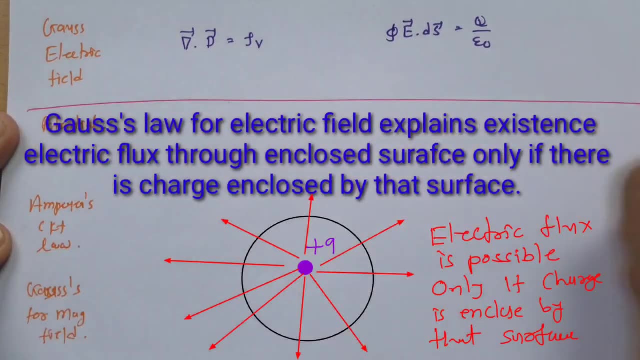 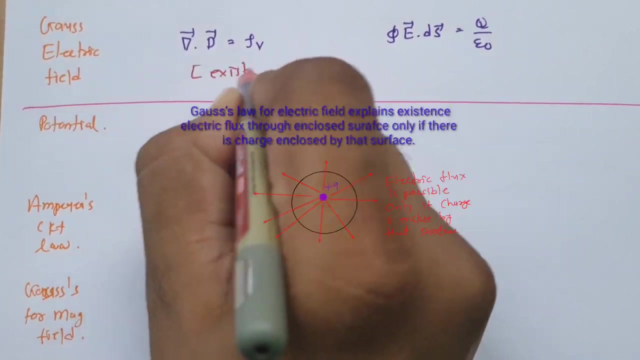 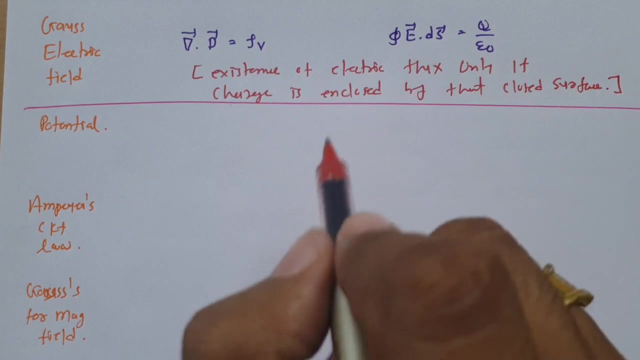 is possible only if charge is enclosed by that surface, right? so let me give you statement here: gauss's law for electric field, that explains existence of electric flux through enclosed surface, is possible only if charge is enclosed by that surface and that electric flux is equals to q by epsilon 0. right now. second, 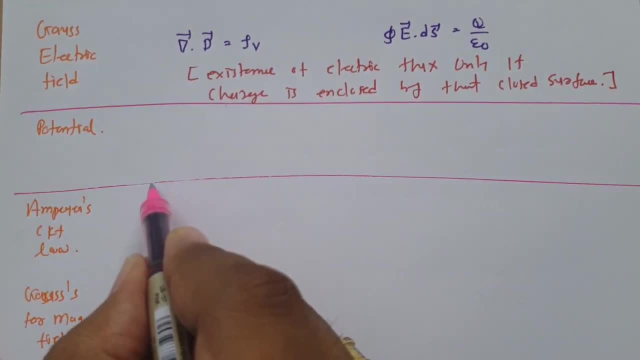 maxwell's equation that is there, based on potential. second maxwell's equation that is there, based on potential now for non-time varying field right now. see by this color, i am explaining everything for non-time varying field right now. see by this color, i am explaining everything for. 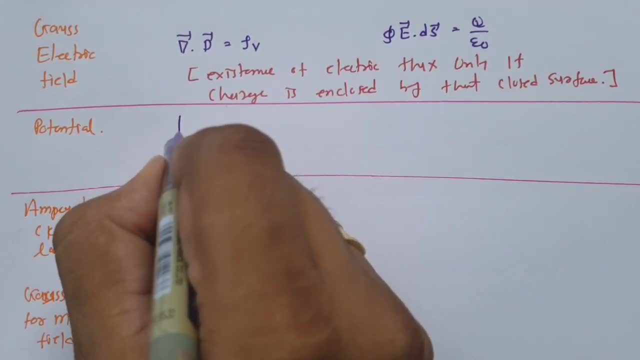 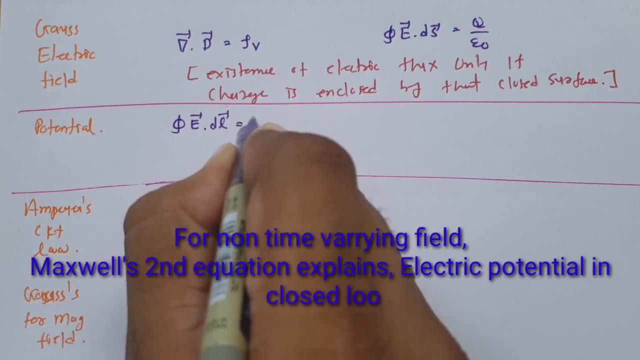 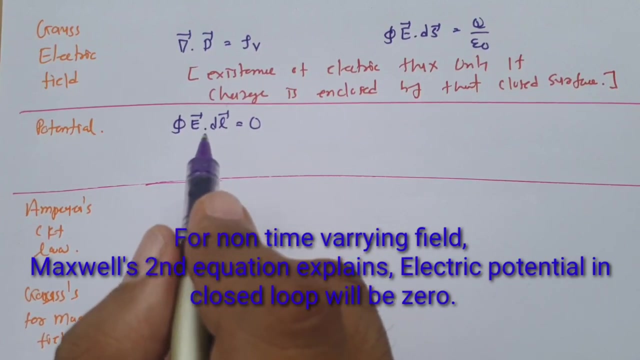 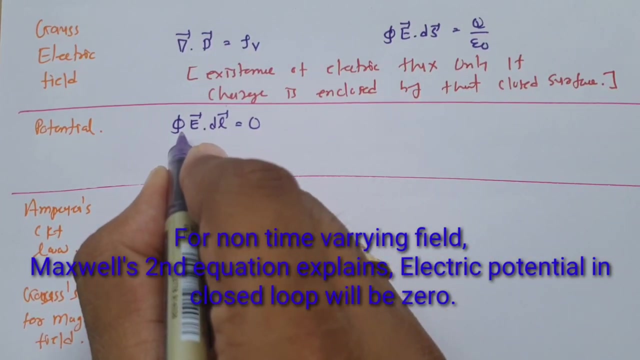 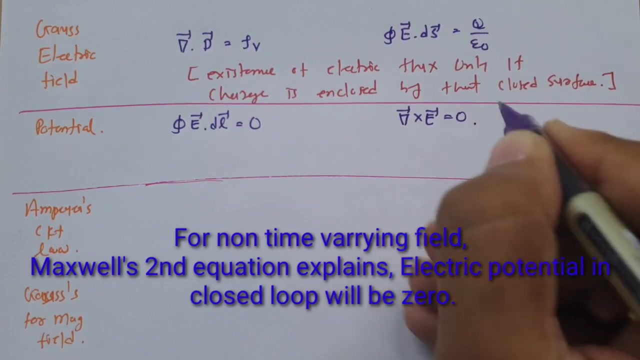 non-time varying field, right. so for non-time varying field, we can say: for closed integration of electric field, that will be zero. so we can say: for closed path line integration of electric field, that is zero and its integral form, that is integration, edl is equals to zero and differential form that is del cross e, that is equals to zero, right. so we can say: 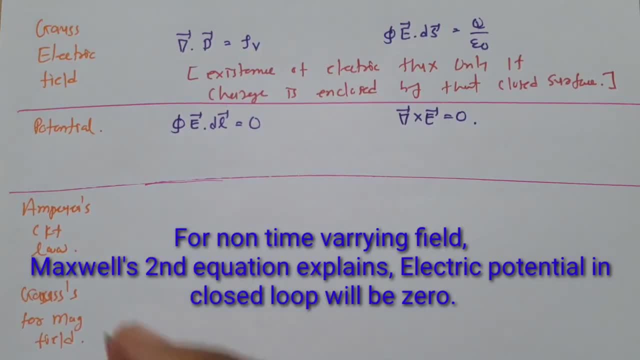 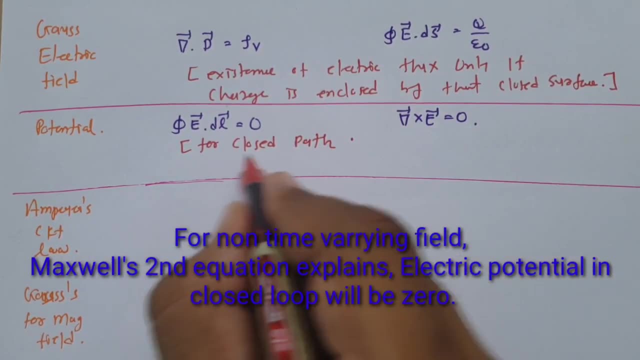 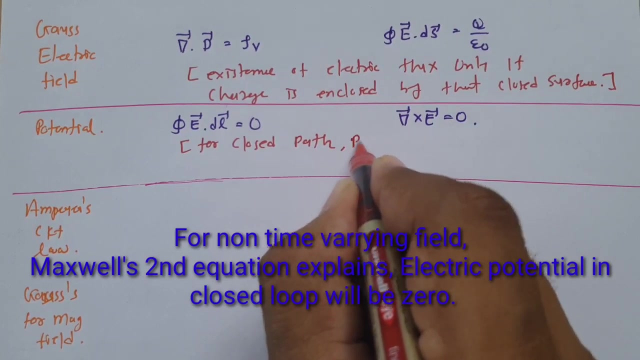 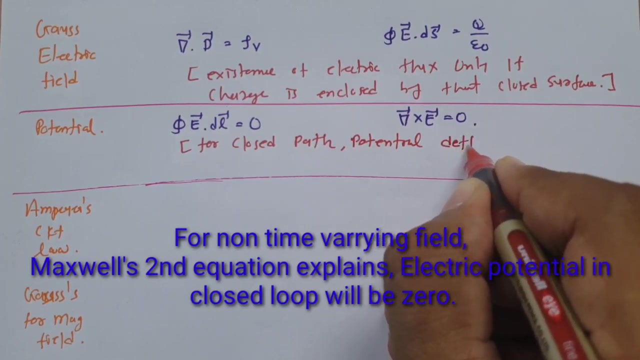 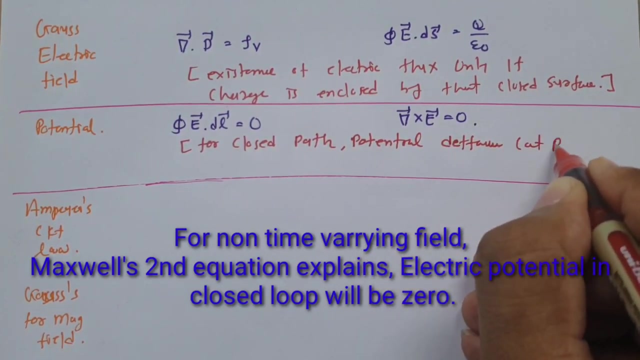 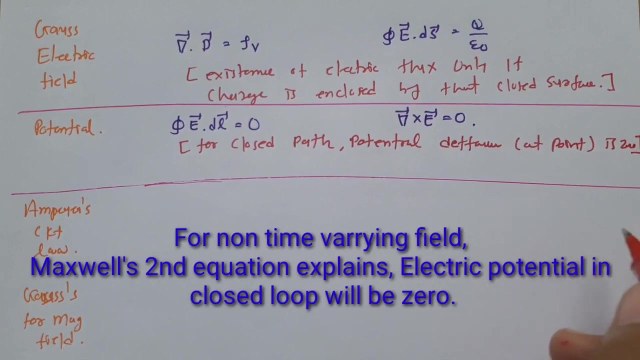 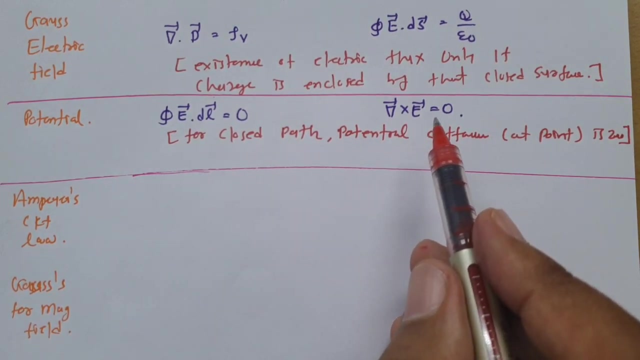 for closed path. for closed path, zero means for closed path. line integration of electric field is what potential? so we can say for closed path, potential potential, potential, potential difference. or one can say potential at point is zero. now, here there is one more equation, that is for time varying field, that we should know, so see, 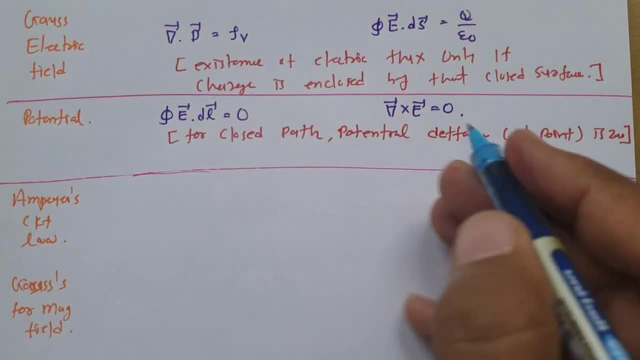 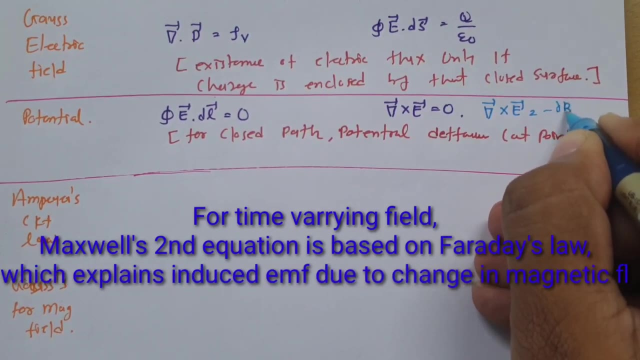 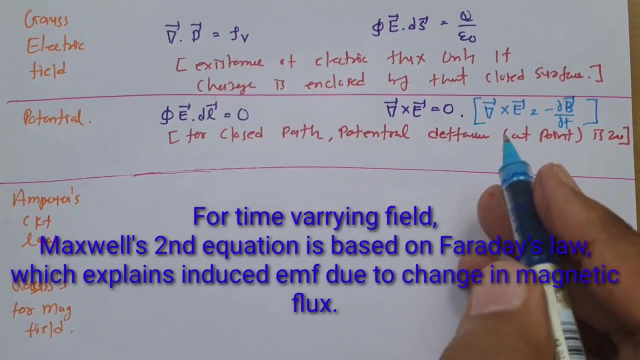 for time varying field, for time varying field. here this equation will get change. for time varying field you will have to say: see del cross, e. that is equals to minus del b by del t, and that is what we are having based on faraday's law. so faraday have explained generation of potential because of rate of change of flux, so we can generate potential. so integration edl is equal to minus del b by del t, and that is what we are having based on faraday's law. so faraday have explained generation of potential because of rate of change of flux, so we can generate potential. so integration edl is equal to minus del b by del t and that is what we are having based on faraday's law. so faraday have explained generation of potential because of rate of change of flux, so we can generate potential. so integration edl is equal to minus del b by del t, and that is what we are having based on faraday's law. so faraday have explained generation of potential because of rate of change of flux, so we can generate potential. so integration edl is equal to minus del b by. 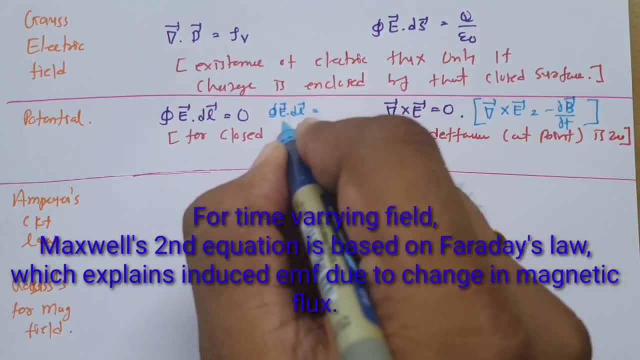 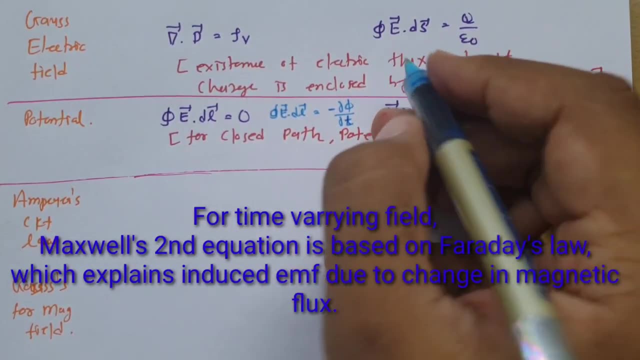 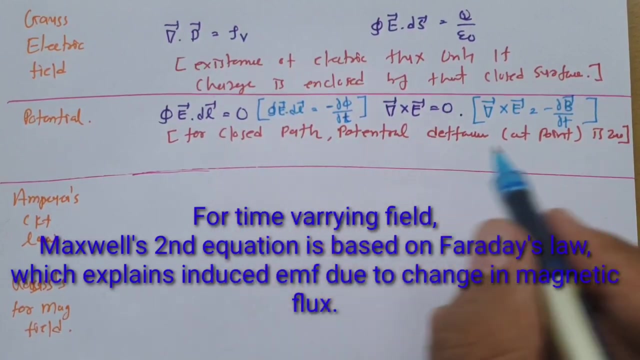 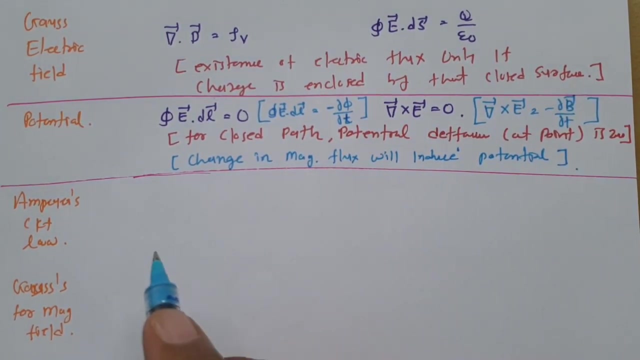 for closed loop integration, edl, that is possible and that is minus change in flux with respect to time, right? so this is what faraday's law, so it explains: change in magnetic flux will induce potential. now see third equation of maxwell that is there, based on ampere circuit law. 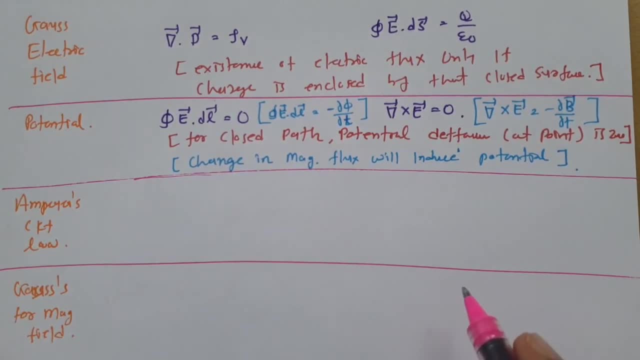 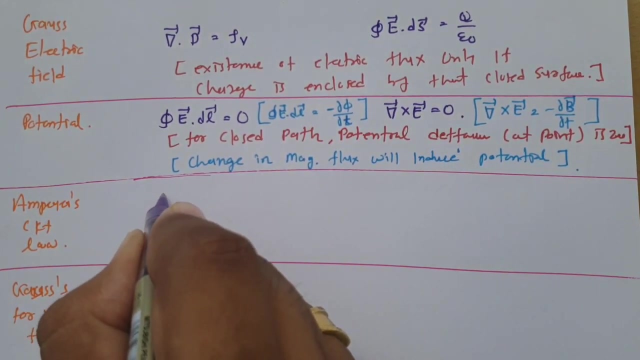 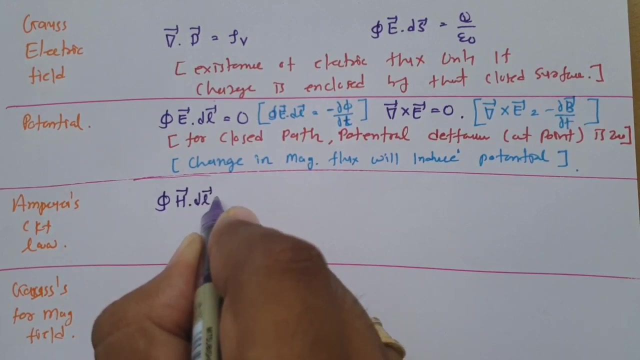 right. so, as we know, ampere circuit law that explains line integration of magnetic field intensity that is equals to current, enclosed by that. so we can say: magnetic line integration of closed line integration of magnetic field intensity that is current, and current is what j dot, ds, ds. 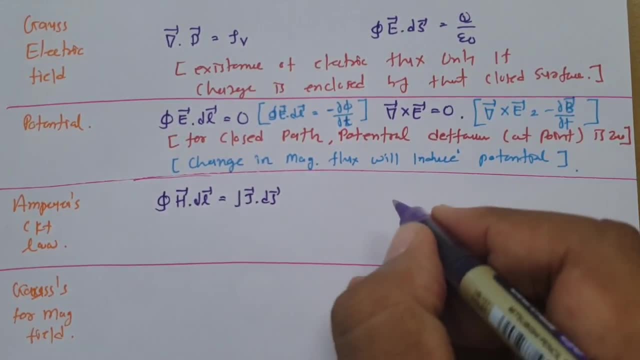 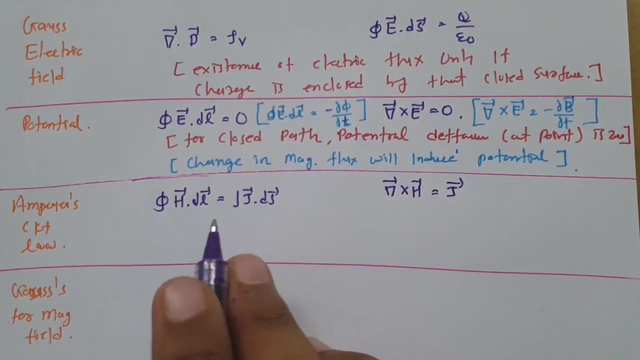 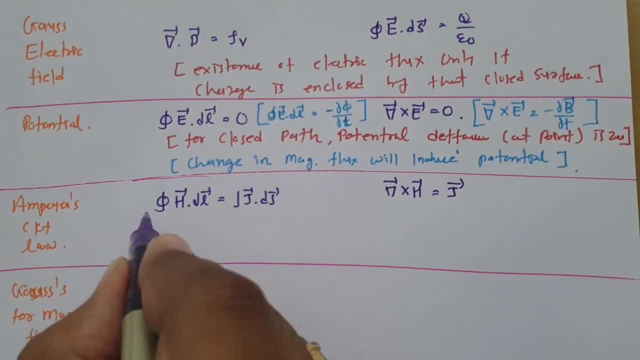 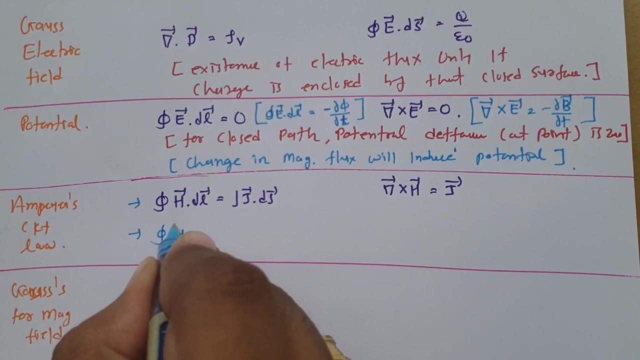 you consider time varying field. so for time varying field, there will be differential current. that will happen. so here, because of differential current, there will be differential current charge density that we need to consider. so for time varying field, i am writing this equation again. so for time varying field, you will be finding that will be integration, hdl, that is. this is for conduction and 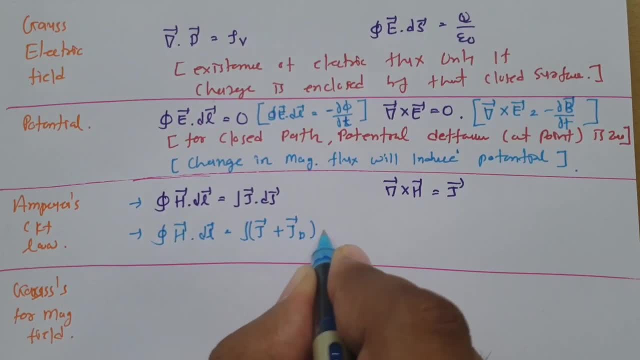 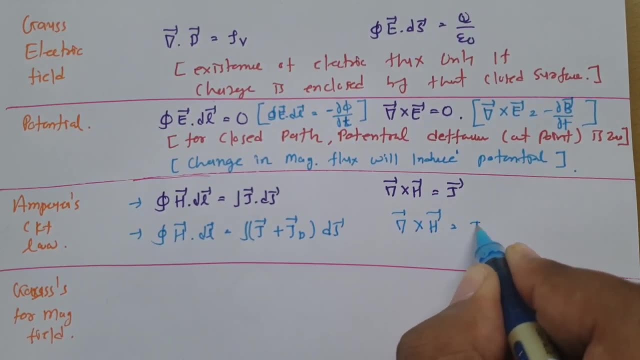 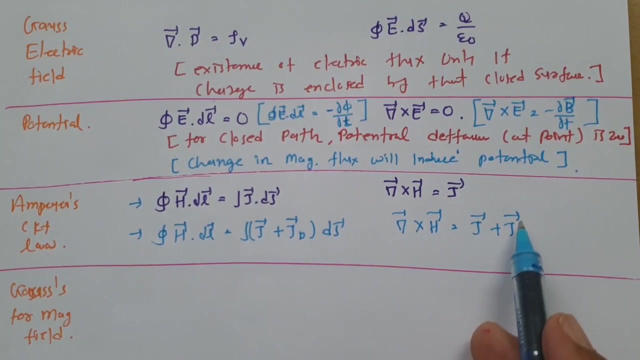 this is for differential current charge density, jd right, and this point form, that is, even changes to del cross. h is equals to j plus jd right. so there will be a generation of differential current charge density because of change in magnetic field, that one can say so for time, varying field, differential current element that will get added. so in terms of 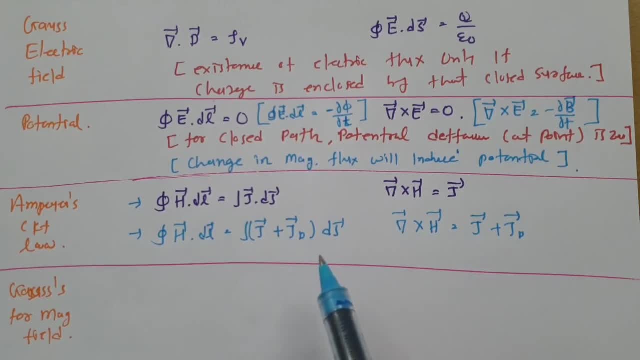 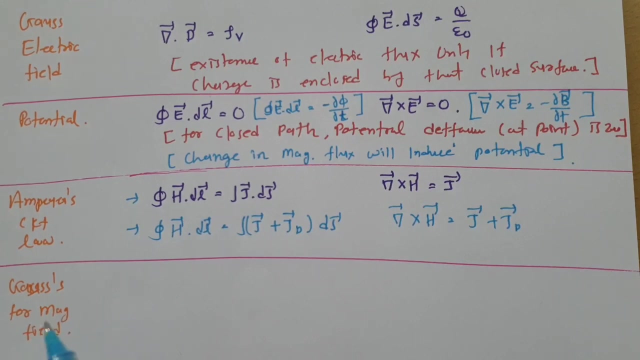 current charge density. we just denote that by jd and for non-time varying field, close line integration of magnetic field intensity that is equals to current. and fourth, Maxwell's equation that is there based on Gauss's law for magnetic field and that Gauss's law for magnetic field is common for time varying as well as non-time varying. 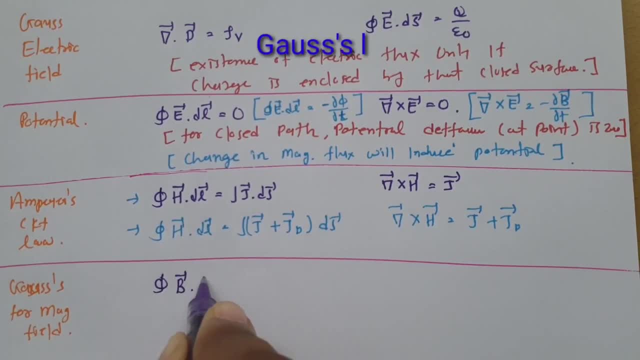 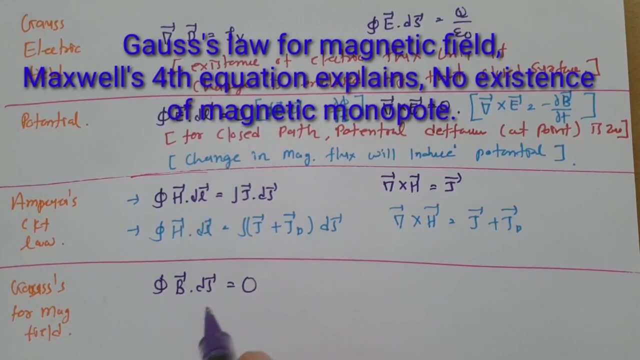 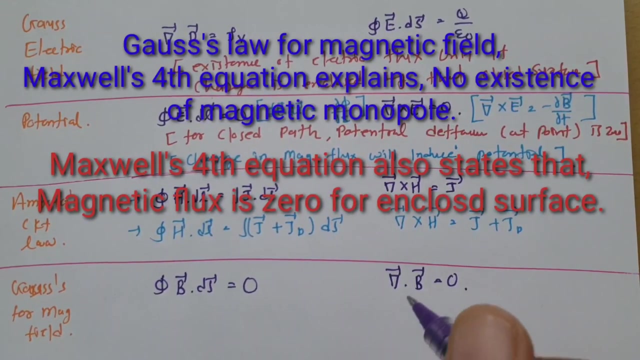 and that is for enclosed surface surface. for enclosed surface, magnetic flux will be zero. for enclosed surface, magnetic flux will be zero. and for point form you can say del dot b, that is equals to zero. and it explains us. isolated magnetic charge does not exist. what does it explains? it explains isolated magnetic. 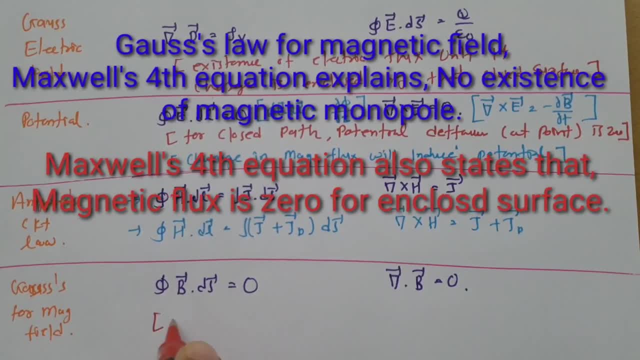 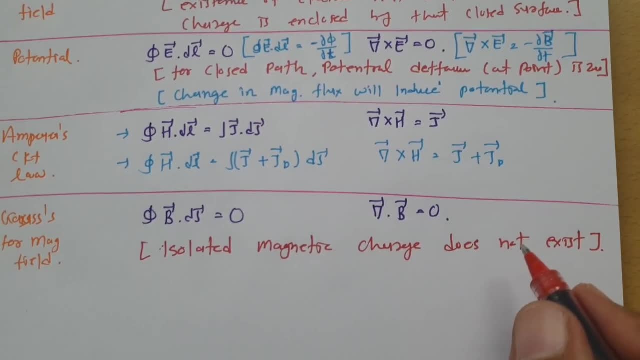 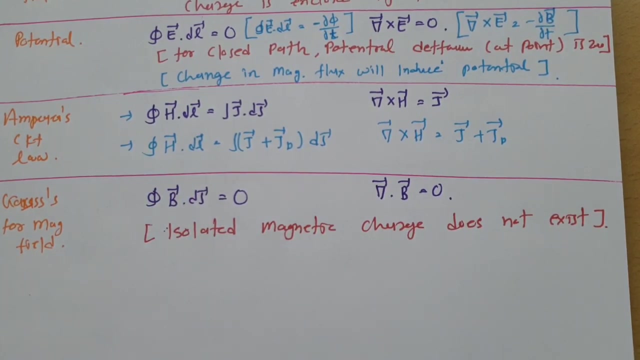 charges does not exist. magnetic, then that voi. so what is the meaning of this see? if you have, if you want to calculate magnetic flux right for enclosed surface like see, I ll consider one enclosed surface over here. let us say this is an enclosed surface, right, and for this enclosed surface it is very compulsory to have isolated magnetic. 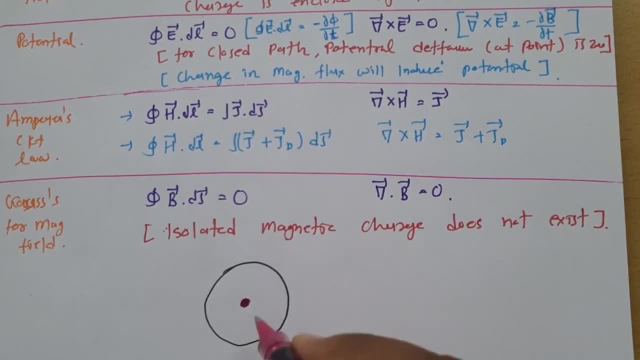 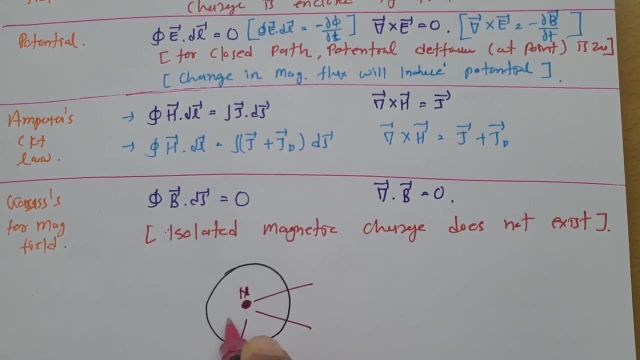 charge? right if i say i have isolated magnetic charge over here. let us say, this is north pole. so for north pole what will happen? magnetic field that will emerge from it. right, so we can say total magnetic flux, that is integration bds over here. but that does not exist, as when you have north pole, then 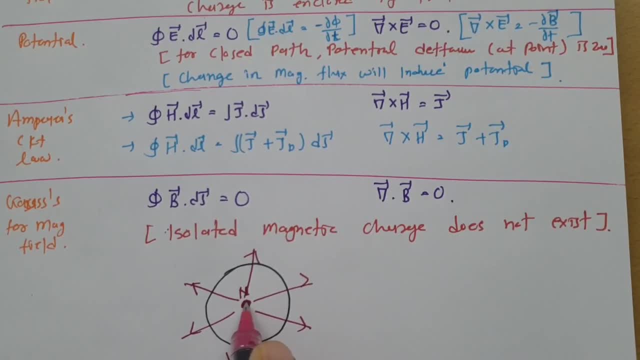 south pole will be there right. so what will happen? you know, like you can see, it does not have only north pole, it has north and south, like this. so when electromagnetic field emerges from north pole, what will happen is like that magnetic field again will come back to south pole, like this: 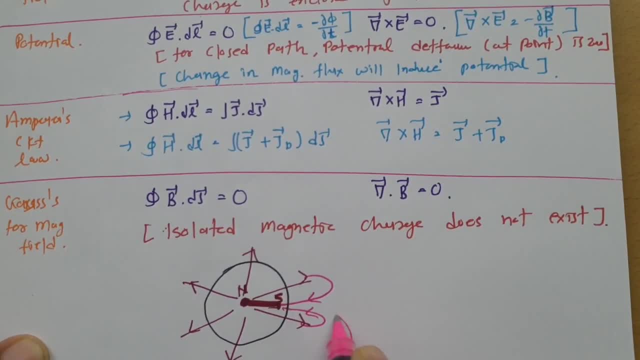 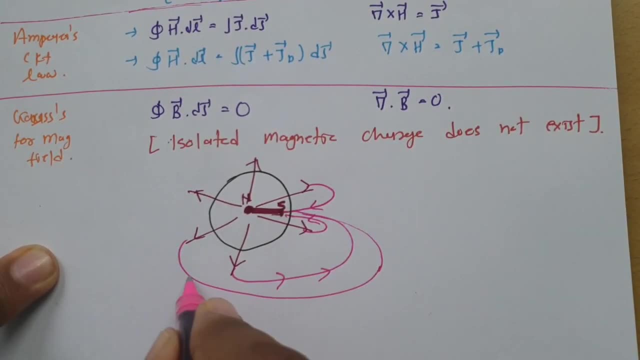 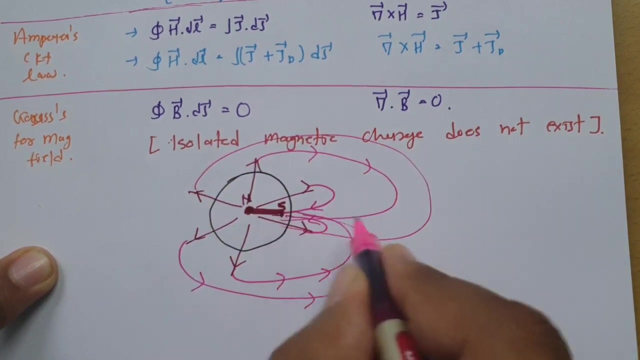 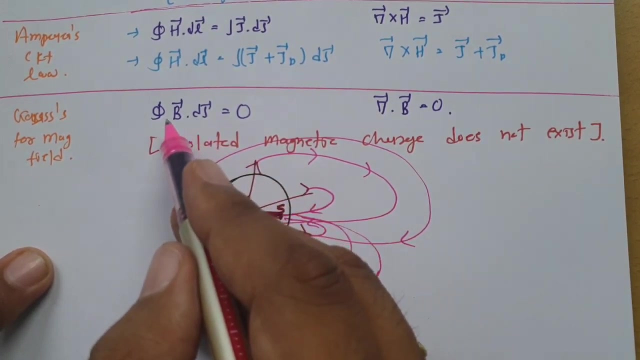 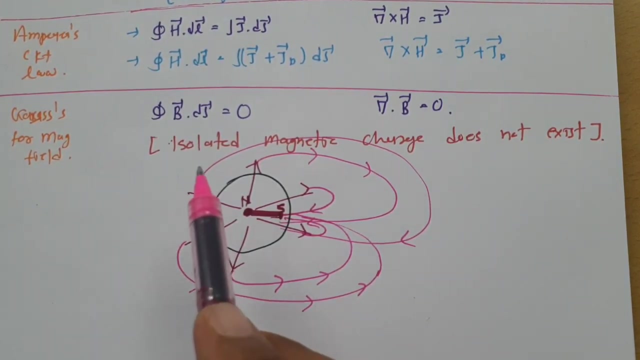 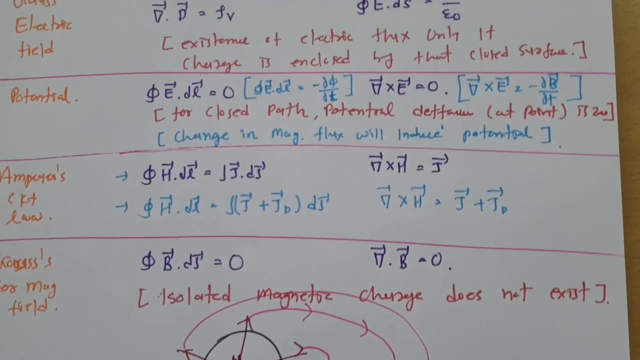 you can see. so what will happen? entering flux is equals to leaving flux and that will make total flux passing through enclosed surface. for magnetic flux it will be zero. so it gives you idea about there is no isolated magnetic charges. so these are the four maxwell's equation. i hope that you